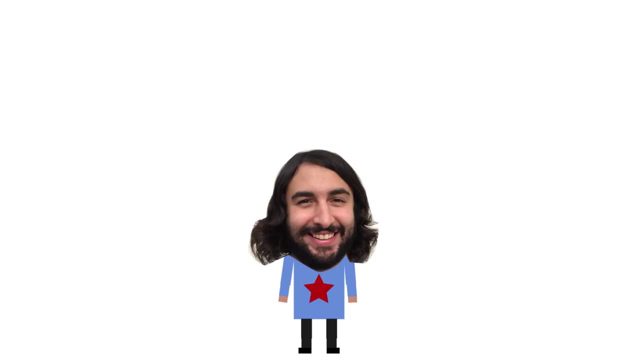 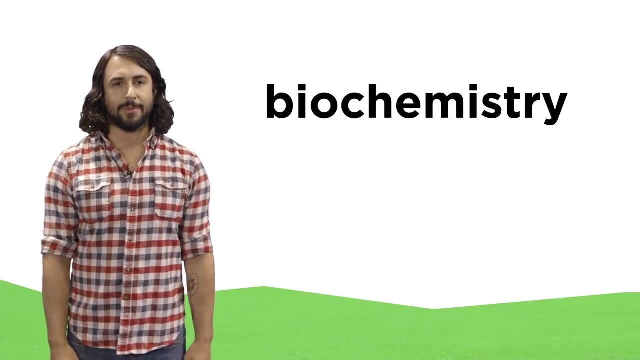 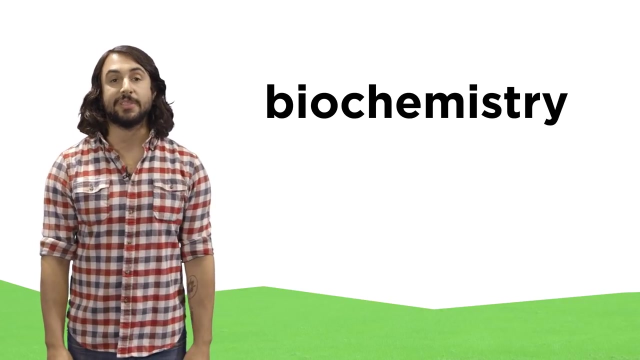 Hey, it's Professor Dave. let's talk about biochemistry. What is biochemistry? Is it biology? Is it chemistry? Well, as you might guess, it's sort of in between, quite literally in terms of size, In the great panoply of the sciences. 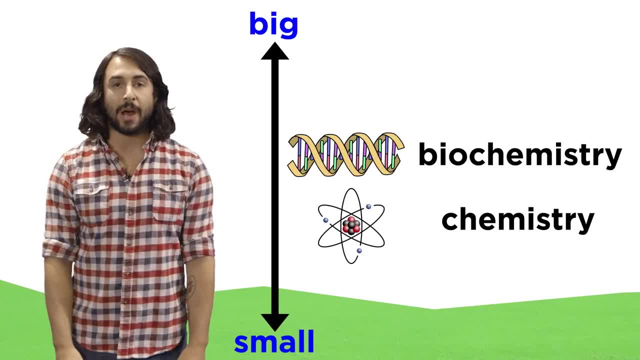 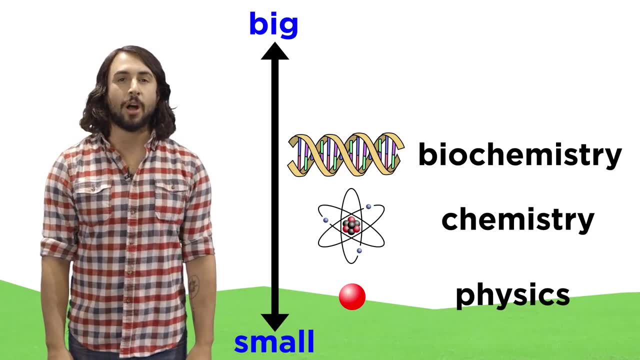 biochemistry sits right here. If we go smaller, we get into small molecules made of just a few atoms, which is chemistry, And even smaller than that. we get to the particles that are even smaller than a single atom, and that's particle physics. If instead, we go much bigger, 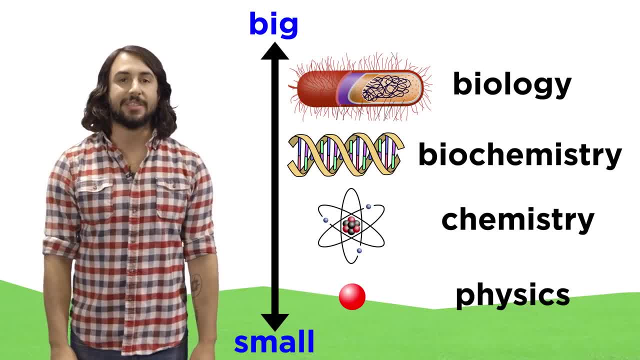 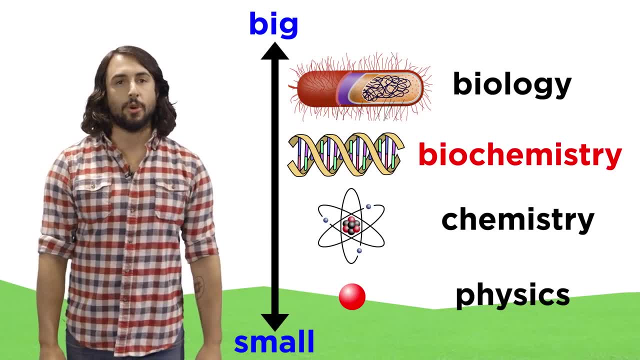 we are looking no longer at individual molecules, but entire cells or parts of a cell. That's biology. Right in between is biochemistry. This is the domain of large biomolecules like proteins and DNA, and the things they can do. Is it important to understand You? 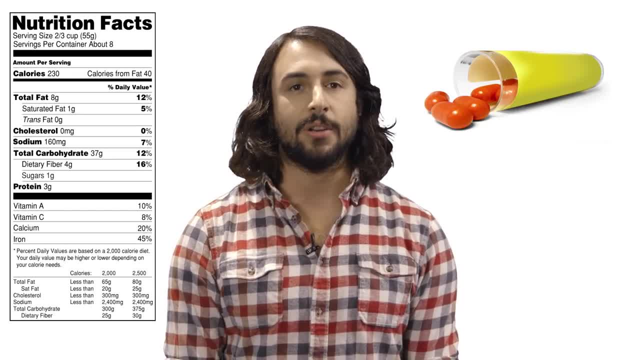 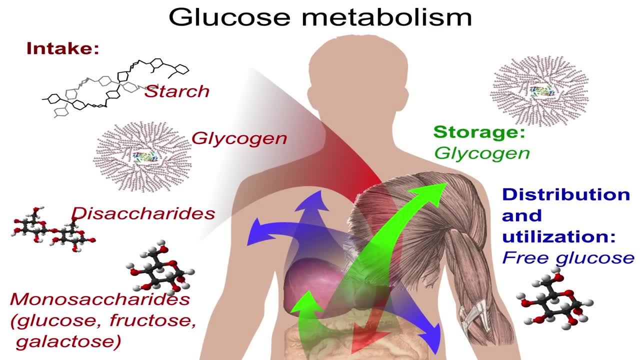 better believe it. Anything that has to do with nutrition, medicine or general health is rooted in biochemistry. That's because nutrition has to do with metabolism, the chemical process by which molecules in your body break down the food you eat. Your health is governed by biochemistry as well. 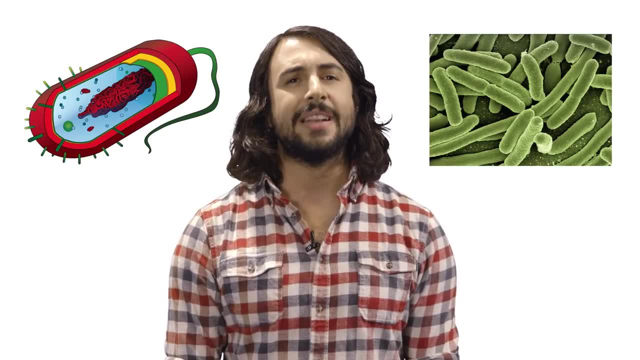 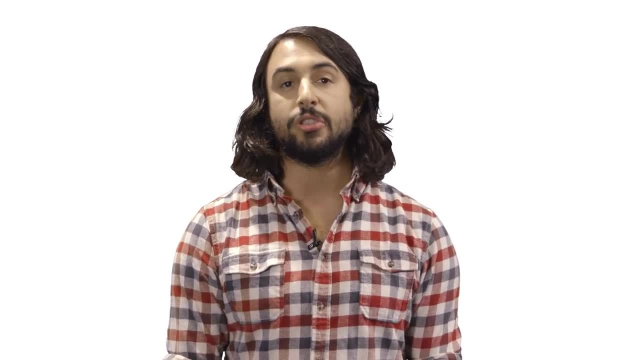 since all diseases have a molecular basis. When you really get down to it, you are just a bunch of molecules, so we need to know what they all do. That's why the domain of biochemistry is so often misunderstood. Everywhere you look, there is a whole bunch of molecules and they all have different. 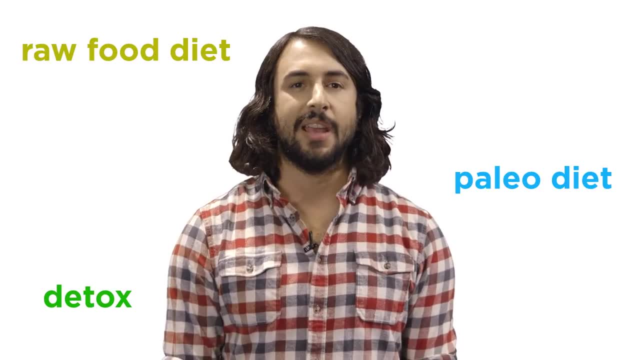 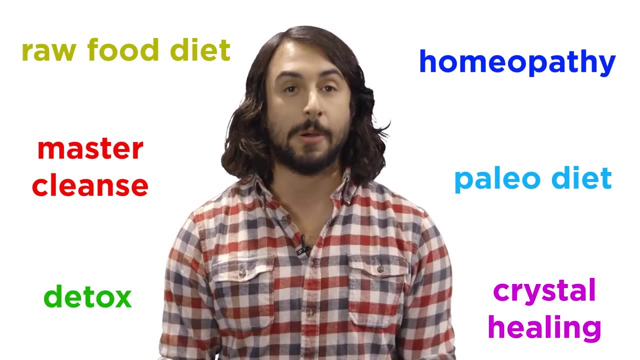 characteristics. There is misinformation, Diet fads, medical hoaxes and pseudoscience from every direction. Many people, when looking at their own health, even try to step away from science completely, opting instead for unsubstantiated alternatives. But this is. 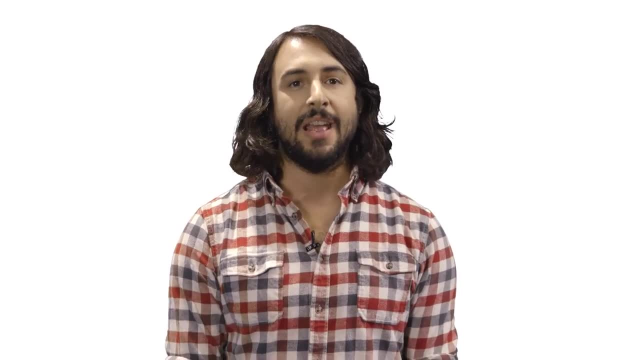 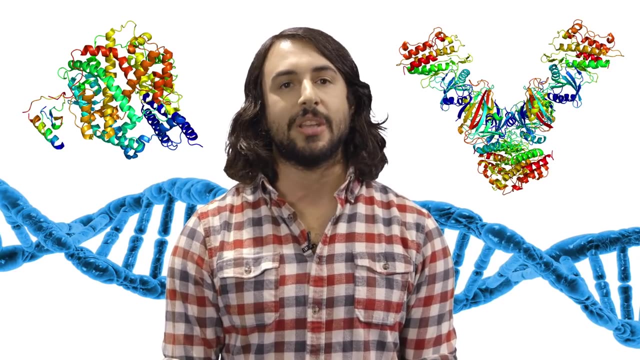 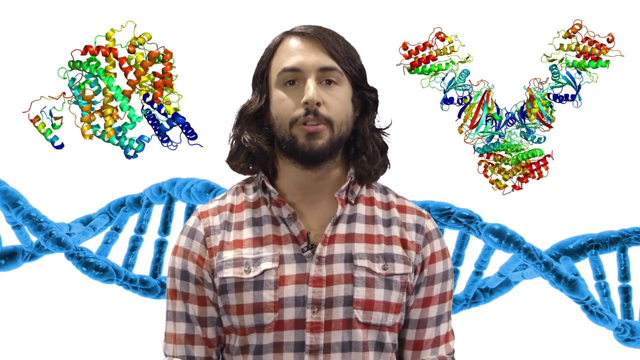 a poor strategy, because the status of everything in your body is governed by large biomolecules like enzymes, receptors and DNA. These are molecules that biochemists understand very well and we all need to learn about them. We all need to learn about them if we want to have any kind of clear picture about what 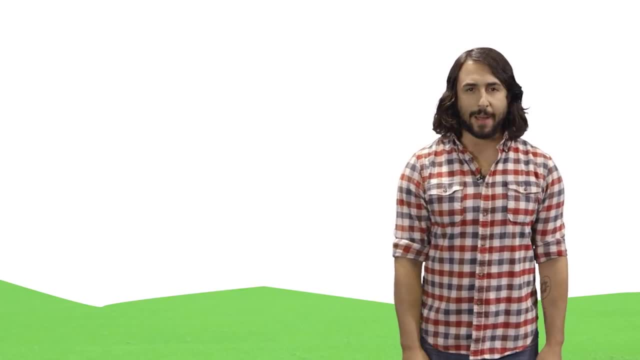 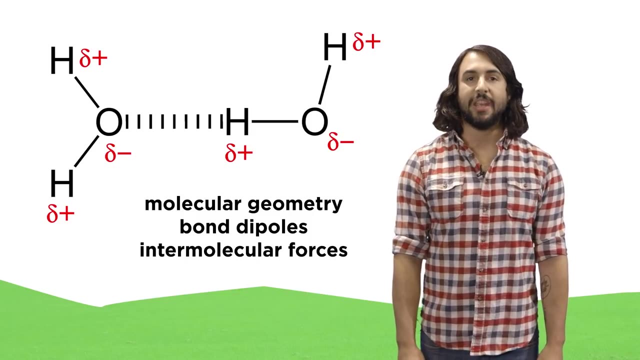 goes on inside the body. Unfortunately, you can't understand biochemistry without understanding the basic chemistry that it breaks down to. What these large biomolecules do is fundamentally the same stuff we learned in general and organic chemistry. It's just a bunch of plus and 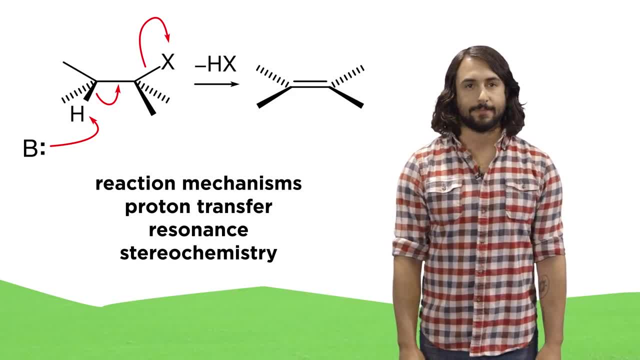 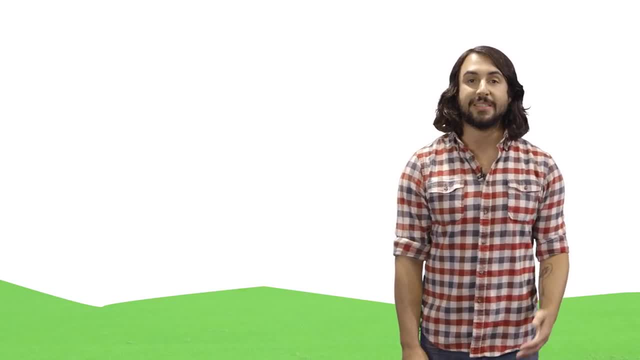 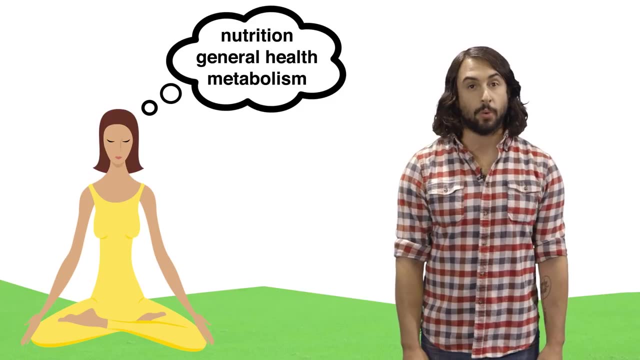 minus charges that make chemical reactions happen. So if you are watching this series to supplement your undergraduate biochemistry course and remember your basic chemistry, you're all set to move forward. If you are someone that just wants to learn more about how the human body works but you haven't learned, 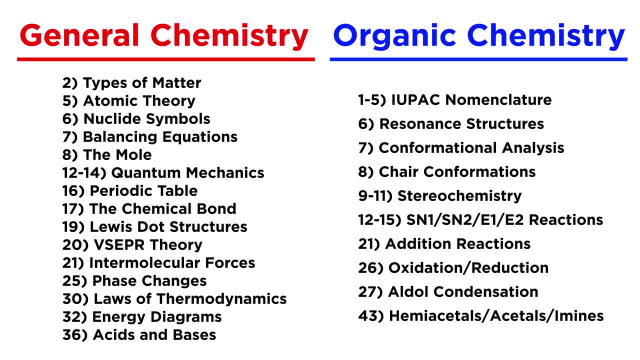 much chemistry. here is a list of other tutorials from my general chemistry playlist and organic chemistry playlist that you really will want to watch first in order for any of this to make sense. I promise this is the bare minimum and I also promise that, if you understand, 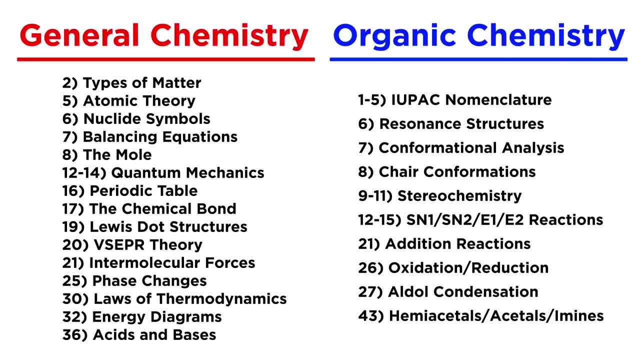 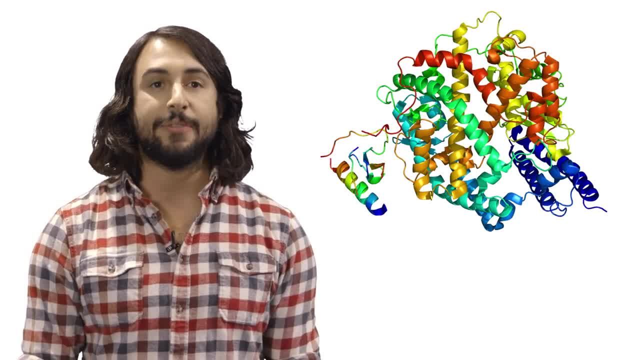 these, everything in this series, will be pretty easy to understand When we see a picture of, say, an enzyme and it looks like a weird tangled blob. we draw it that way to save time because there are hundreds or even thousands of atoms in it. 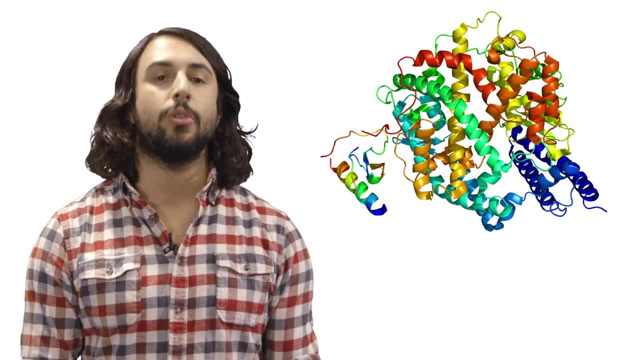 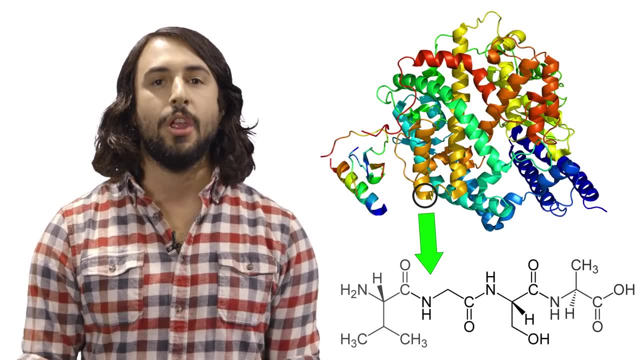 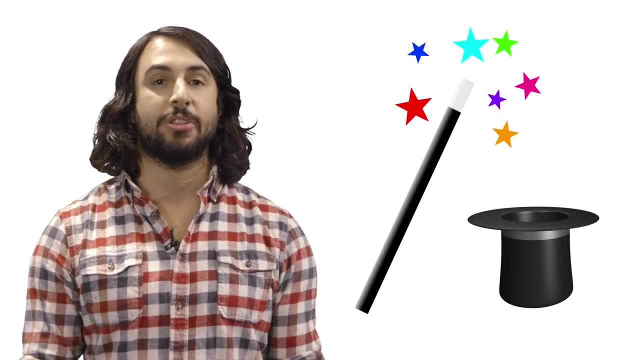 which would be impractical to draw out individually using the line notation we are familiar with. But we absolutely must be able to understand this enzyme on the molecular level so we can know what functional groups it's made of and how it does. basic chemistry Otherwise. 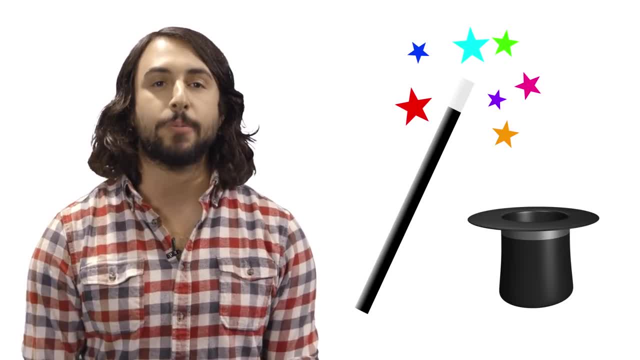 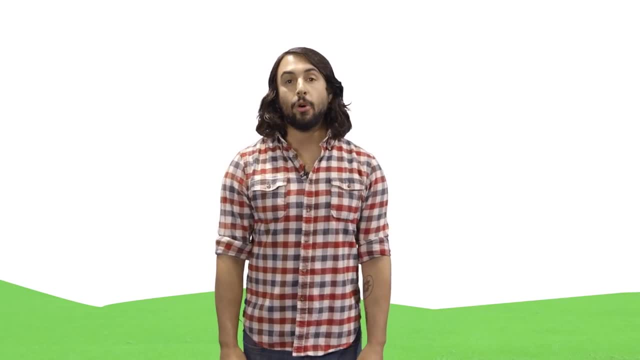 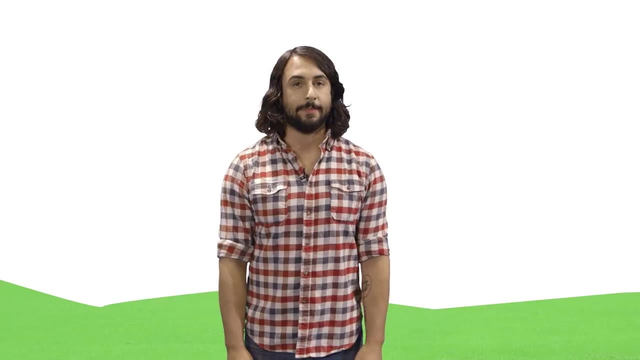 chemistry seems like magic, But it's not. it's just many surprisingly simple chemical reactions, even if they are applied in complex ways and on huge molecules. My goal with this series is to focus on the basic concepts of biochemistry and illuminate them for the student and the common viewer alike. I may occasionally mention details. 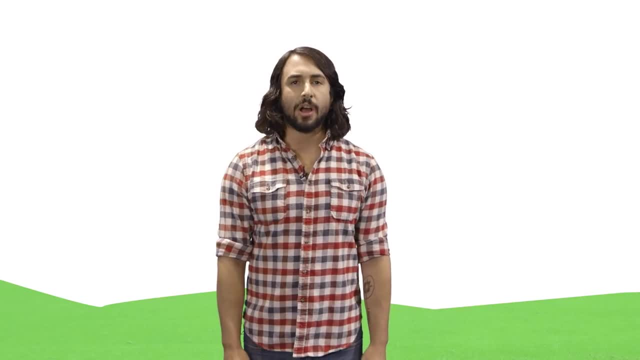 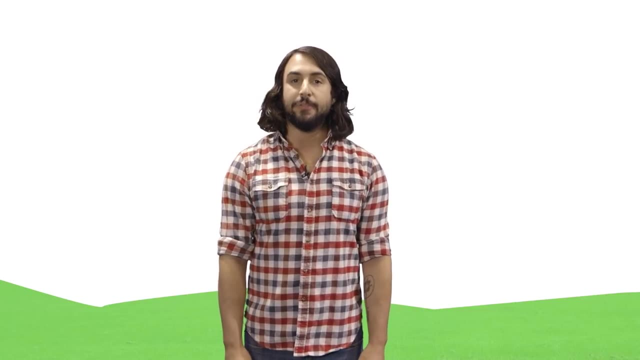 that aren't that important to non-students, and I also may gloss over some of the more technical details. This is in hopes of keeping everyone engaged, But for anyone who might be viewing these tutorials, if you focus on gaining the big picture of all these biochemical 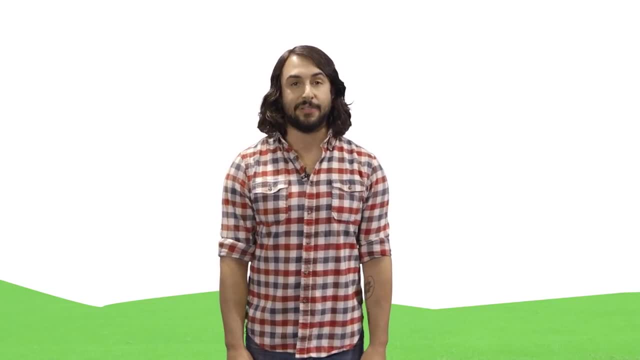 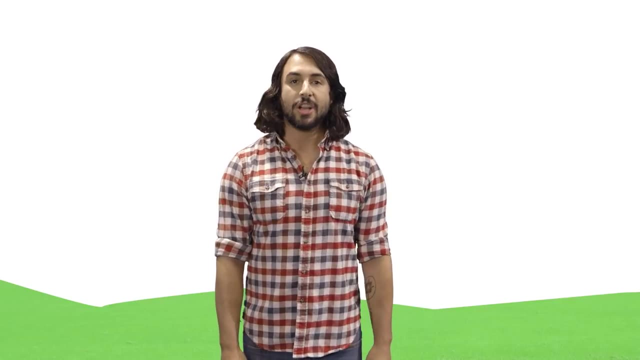 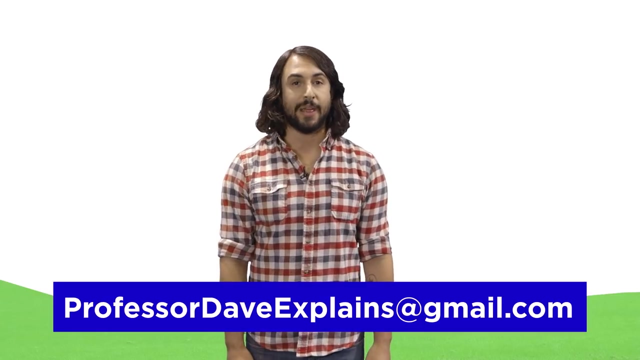 processes working together to create the complexity of life, you will emerge much wiser at the end of the playlist. Whatever you do, don't get discouraged. watch more than once if you need to and, as always, feel free to email me with any questions you might have at professordaveexplains. 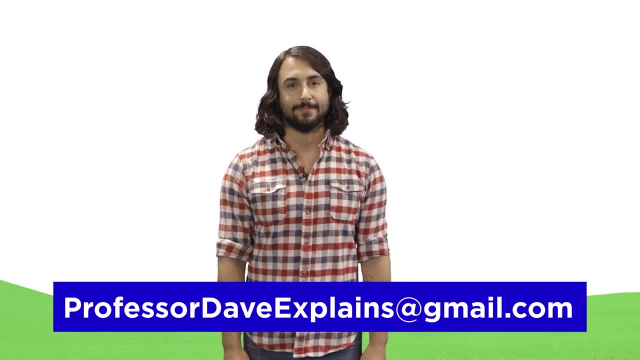 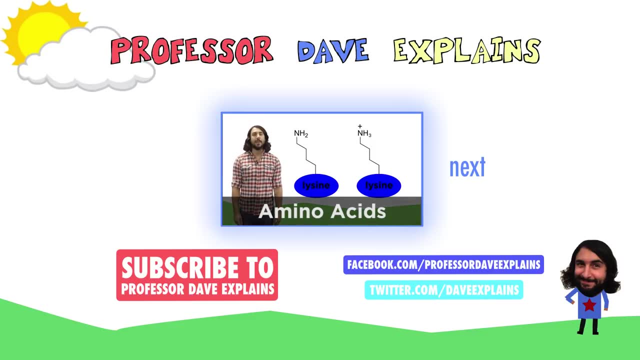 at gmail dot com. Now let's learn some biochemistry. Thank you very much for watching and I'll see you next time.